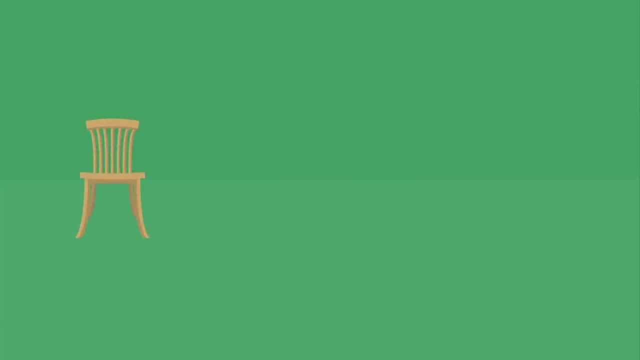 So let's see if there's a quicker way. Let's start with the first person, Going from the beginning again. you can see that each of the four initial choices for the first chair leads to three more possible choices for the second chair, And each of those choices leads to two more for the third chair. 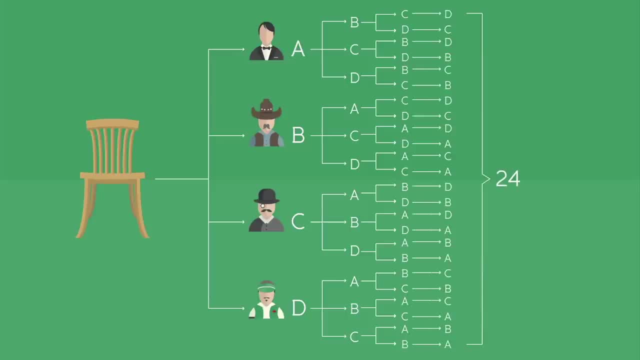 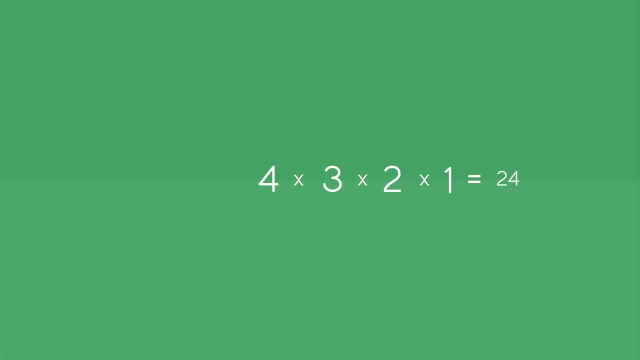 So instead of counting each final scenario individually, we can multiply the number of choices for each chair 4 times 3 times 2 times 1, to achieve the same result of 24.. An interesting pattern emerges. We start with the number of objects we're arranging. 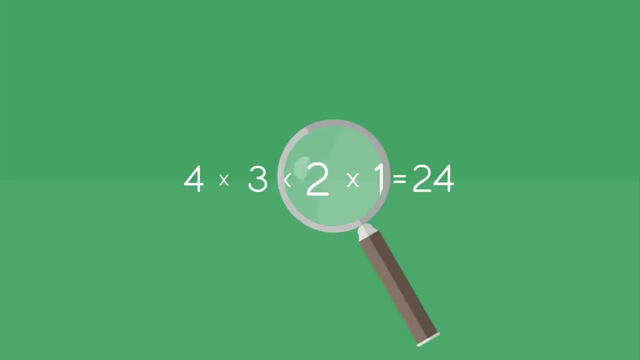 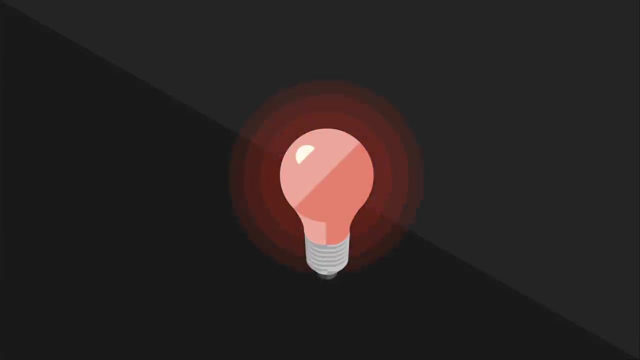 4 in this case, and multiply it by consecutively smaller integers until we reach 1.. This is an exciting discovery, so exciting that mathematicians have chosen to symbolize this kind of calculation, known as a factorial, with an exclamation mark. 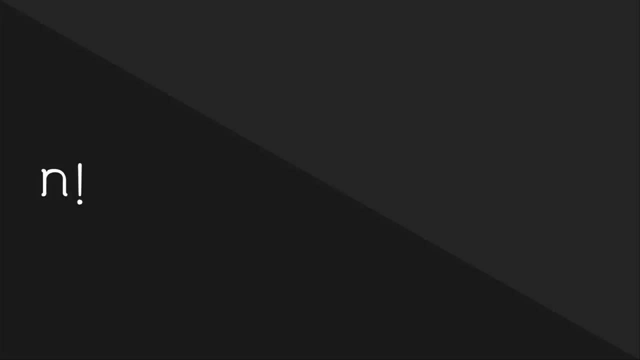 As a general rule, the factorial of any positive integer is calculated as the product of that same integer and all smaller integers down to 1.. In our simple example, the number of ways four people can be arranged into chairs is written as 4 factorial. 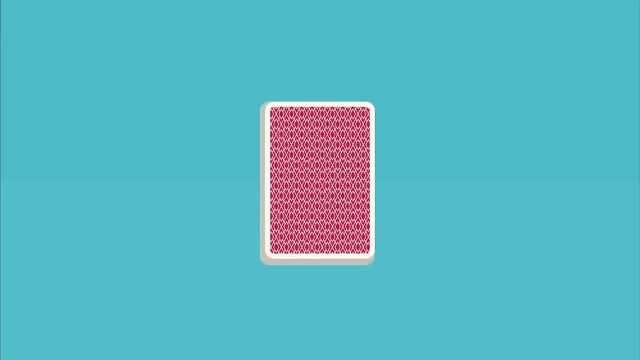 which equals 24.. So let's go back to our deck. Just as there were four factorial ways of arranging four people, there are 52 factorial ways of arranging 52 cards. Fortunately, we don't have to calculate this by hand, Just enter the function into a calculator. 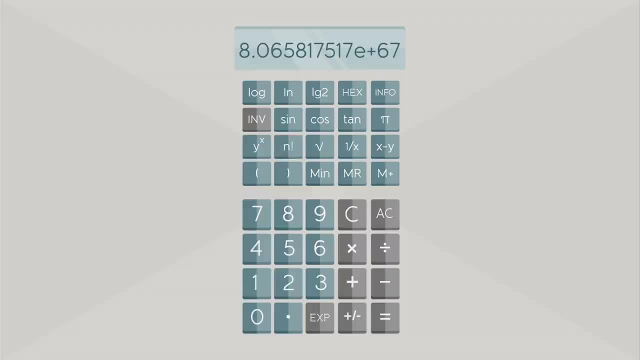 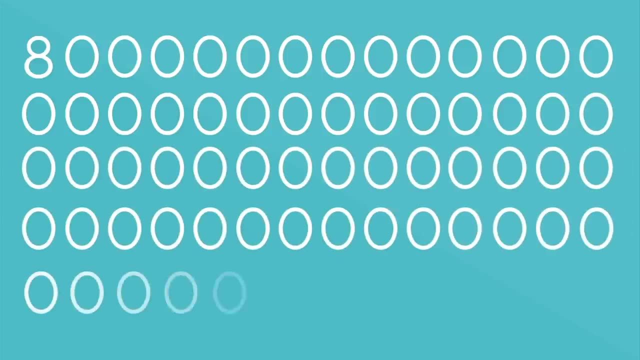 and it will show you that the number of possible arrangements is 8.07 times 10 to the 67th power, or roughly 8, followed by 67 zeros. Just how big is this number? Well, if a new permutation of 52 cards were written out every second, 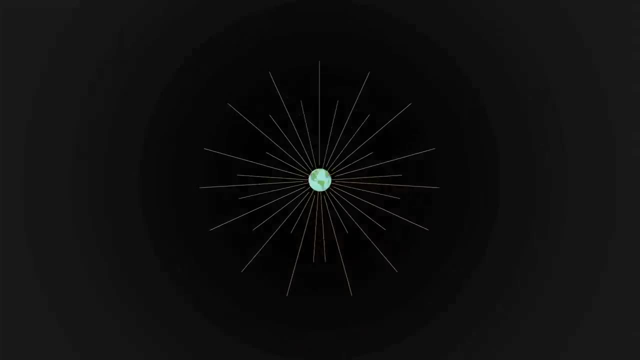 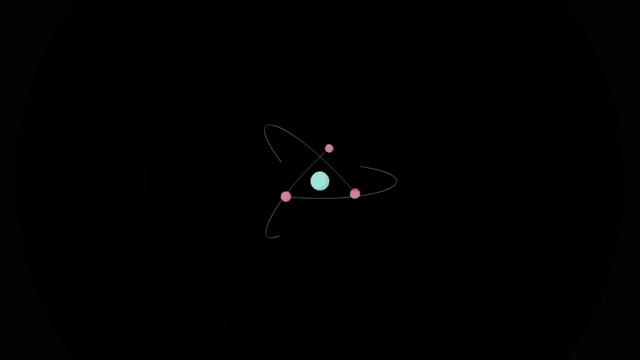 starting 13.8 billion years ago, when the Big Bang is thought to have occurred, the writing would still be continuing today and for millions of years to come. In fact, there are more possible ways to arrange this simple deck of cards than there are atoms on Earth. 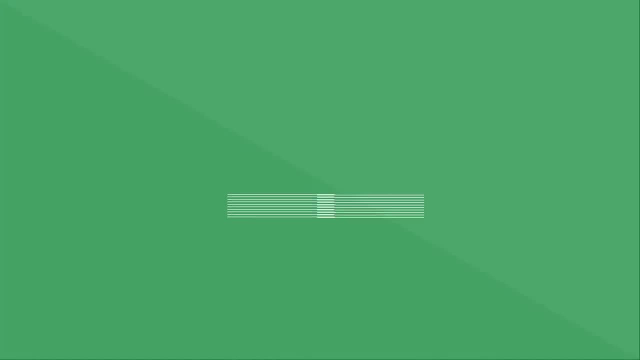 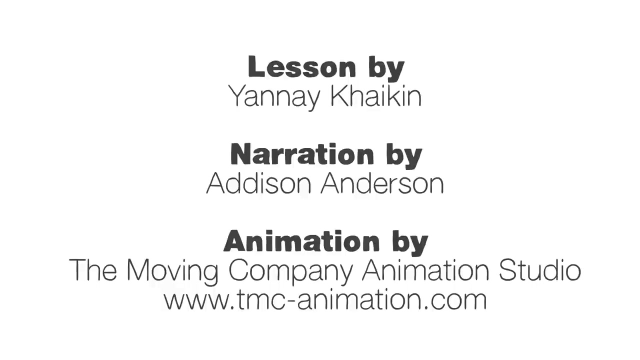 So the next time it's your turn to shuffle, take a moment to remember that you're holding something that may have never before existed and may never exist again. Subtitles by Subtitle Workshop.